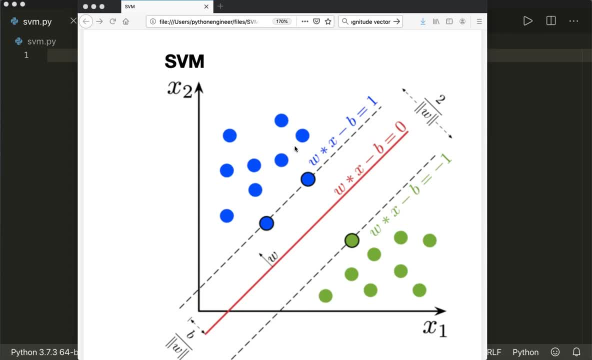 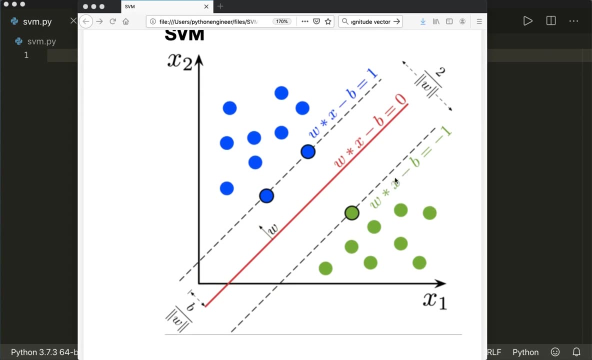 be greater or equal than one for our class plus one. So all the samples here must lie on the left side of this equation, or this line here, And all the samples of the class minus one must lie on the right side from this equation. So if we 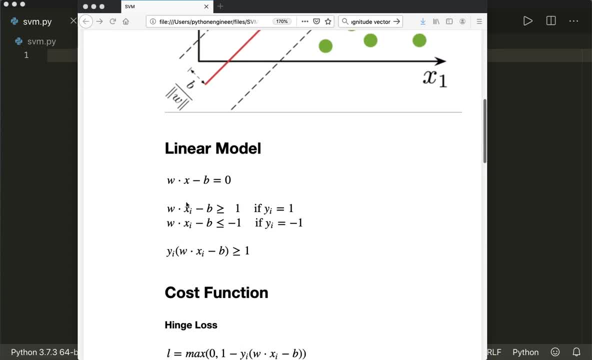 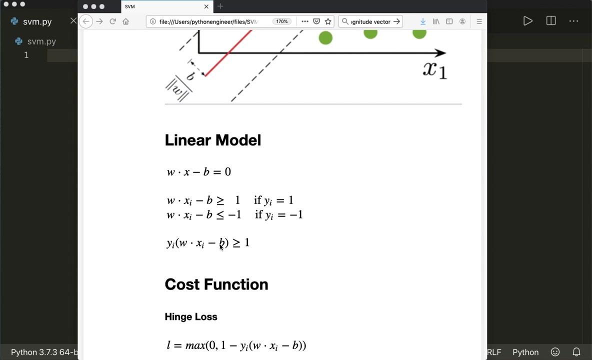 put this mathematically, then we should. it must satisfy w times: x minus b should be greater or equal than one for class one, or it should be less or equal than minus one for class minus one. So if you put this in only one equation, then we multiply our linear function with the class label and this should: 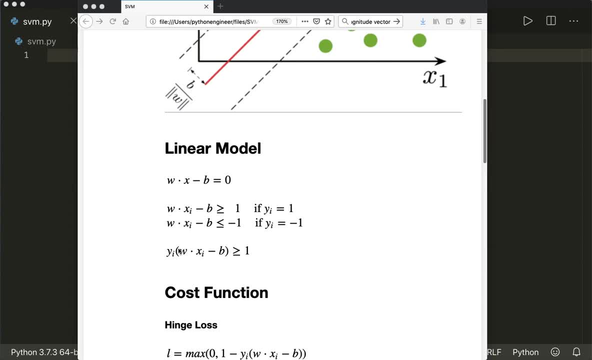 be greater or equal than one. So this is the condition that we want to satisfy. And now we want to come up with the w and the b, So our weights and the bias, And for this we use the cost function and then apply gradient. So we want to have a constant v Now, because 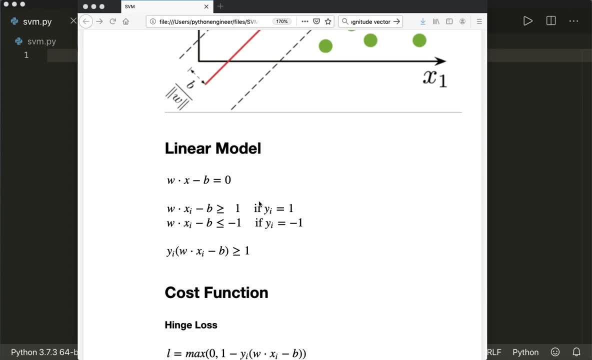 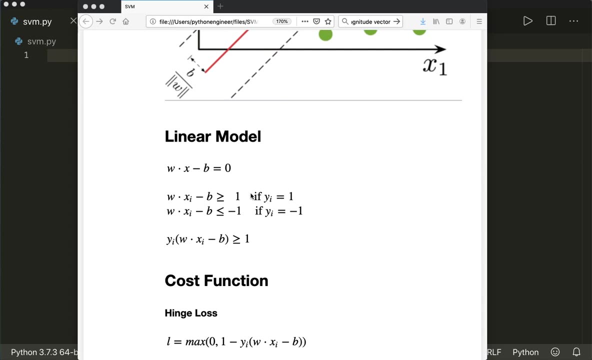 gradient descent. So if you're not familiar with gradient descent already, then please watch one of my previous tutorials, for example the one with linear regression. there I explained this a little bit more in detail. So now let's continue. So we use the user cost function. 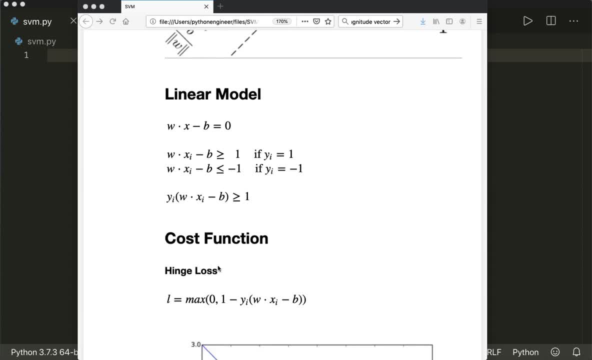 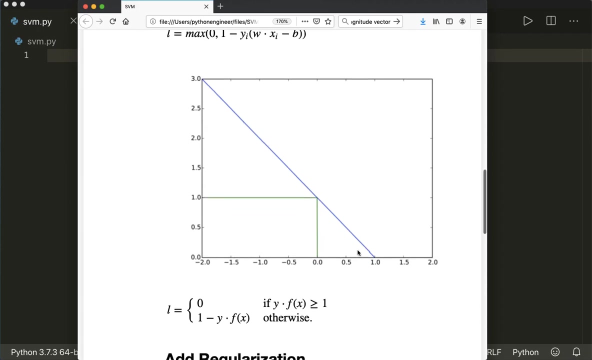 here, And in this case we use the hinge loss, And this is defined as the maximum of zero and one minus. And here we have our condition, why I times our linear model. So what this means is if, if we plot the hinge loss, and here the blue line is the hinge loss. So 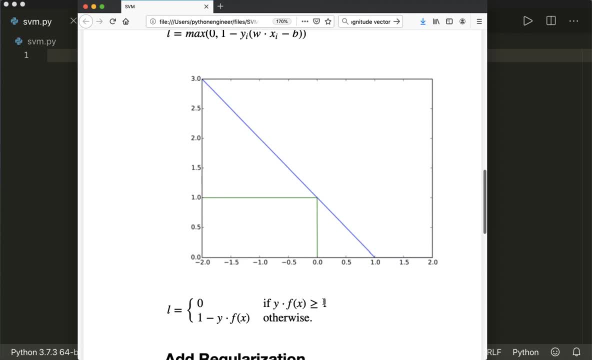 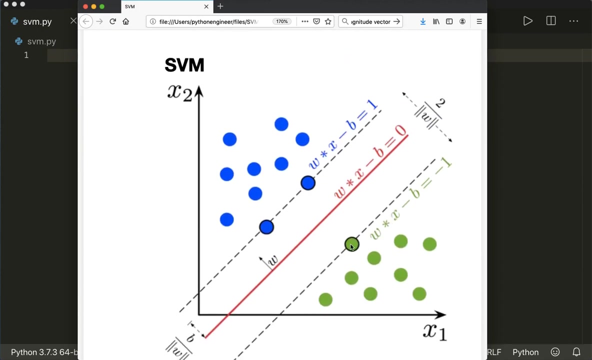 this is either zero if y times f is greater or equal than one. So if they have the same sign, then it's zero. And so if they- Yeah, if they are correctly classified and are larger than one, then our loss is zero. So this means, if we have a look at this image again, if for the green class, if it's- 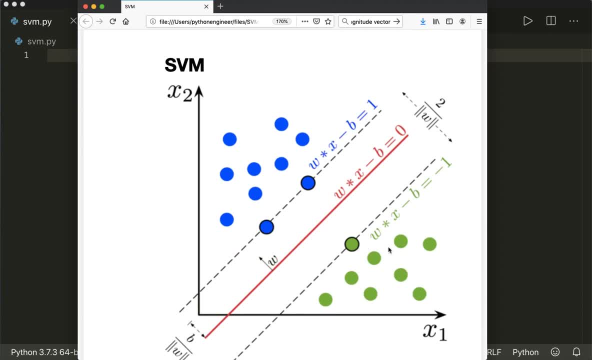 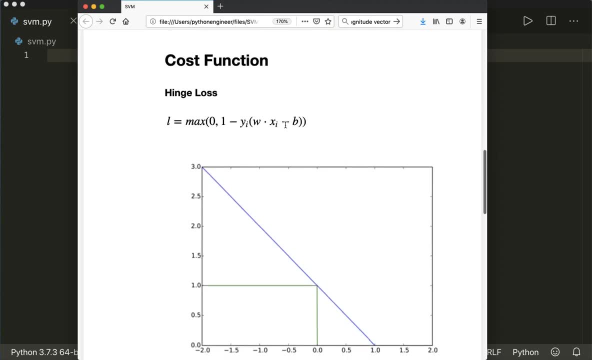 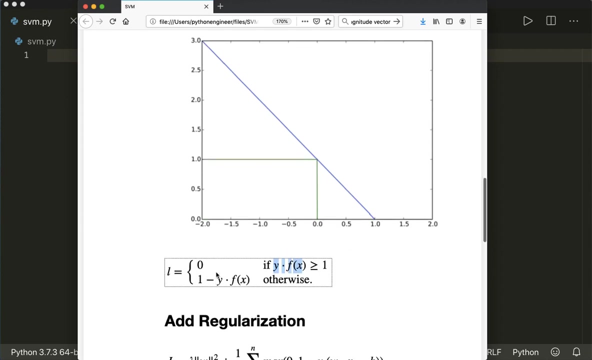 if it lies on this side, then it's zero, And for the blue class, if it lies on this side, then it's also zero, And otherwise, and then we have a linear function. So the further we are away from our decision boundary line, the higher is our loss, And so this is one. 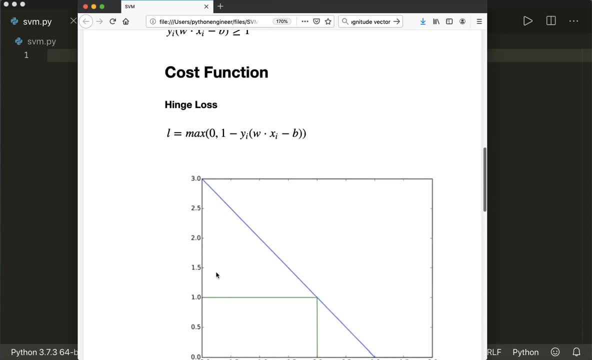 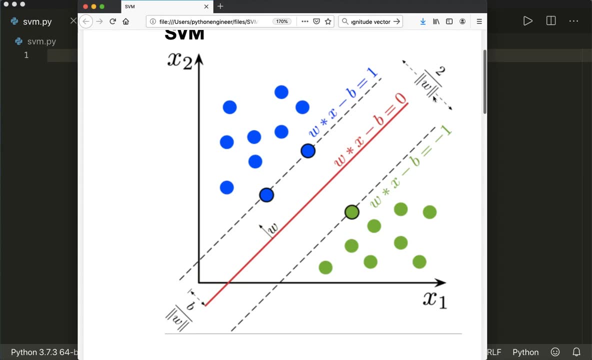 part of our cost function And the other part is, as I already said, we want to maximize the margin here. So between these two classes, and the margin is defined as two over the magnitude of w, So this is dependent from our weight, dependent on our weight vector. So we want to maximize this And therefore, 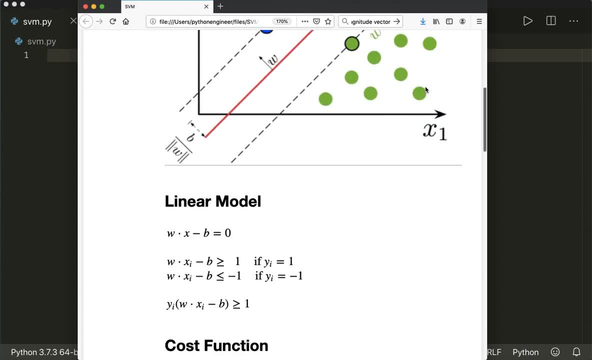 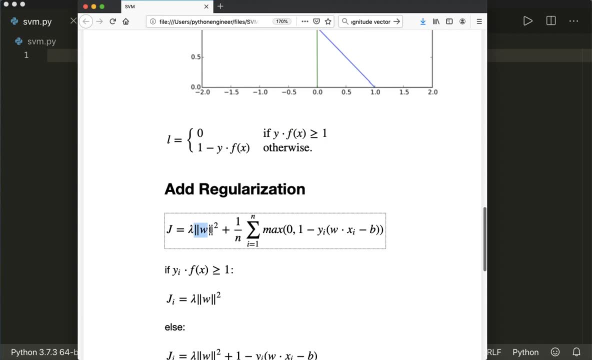 we want to minimize the, the magnitude, So we put this or add this to our cost function, So we also put this term, the magnitude of w, to the power of two times a lambda parameter, And then here we have our hinge loss. So the lambda parameter tries to find a trade off between these two terms. 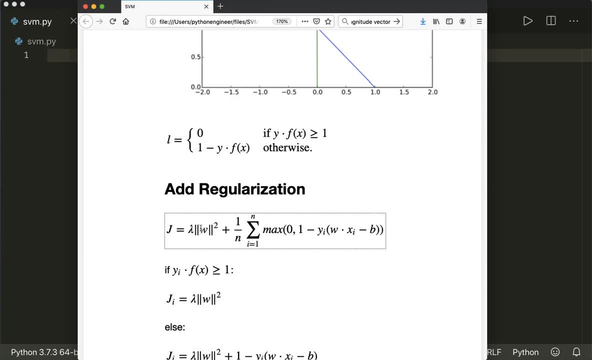 So we, it says, basically says which is more important? So we want to, of course, we want to have the right classification, we want to lie on the correct side of our lines, But we also want to have the, the line such that the margin is is maximized. So yeah, so if 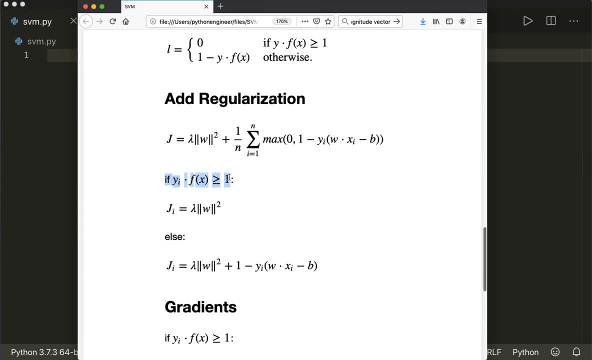 you look at the two cases, if our, if we are on on the correct side of the line, so if y i times f on x, f of x is greater or equal than one, then we, simply we only have this term because this is the hinge- loss is zero And 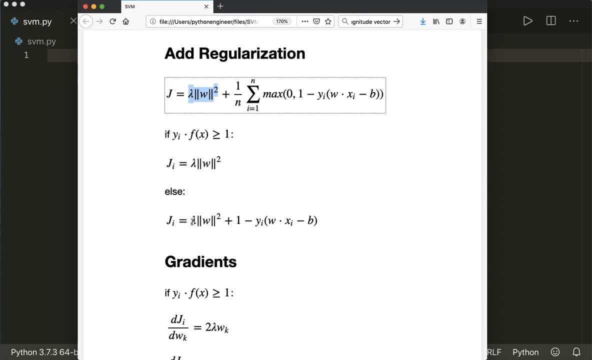 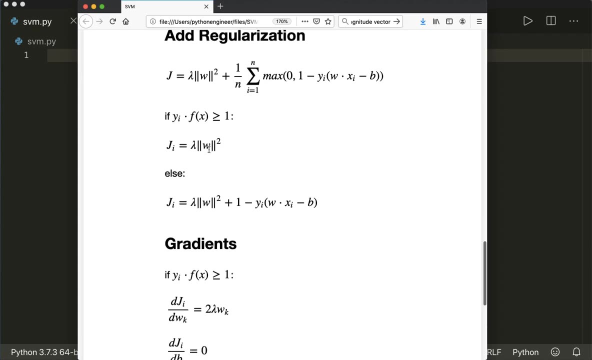 otherwise, then our cost function is this: here And now we want to minimize that. So we want to get the derivatives, or the gradients, of our cost function. So in the first case, if we are greater or equal than one, our derivative is only, is two times lambda, times w. So and 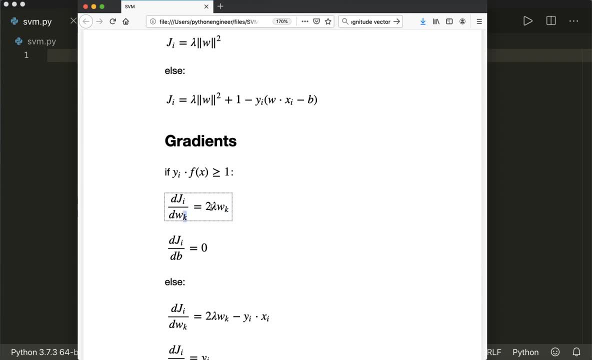 here we only look at one component of our w, so we get rid of the magnitude And then the derivative with respect to the b is zero. So please double check that for yourself. here I will not explain the derivatives and details, And in the other case, so if, if y i times, 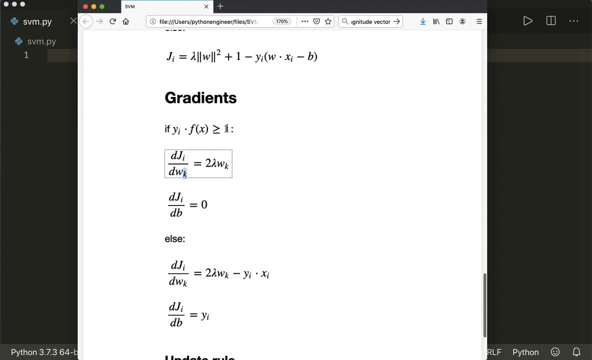 f on x is not greater or equal than one, then our derivative with respect to the w is this equation here, And the derivative with respect to the w is this equation here, And the derivative with respect to our bias is only y, i. So again, please double check that for yourself And 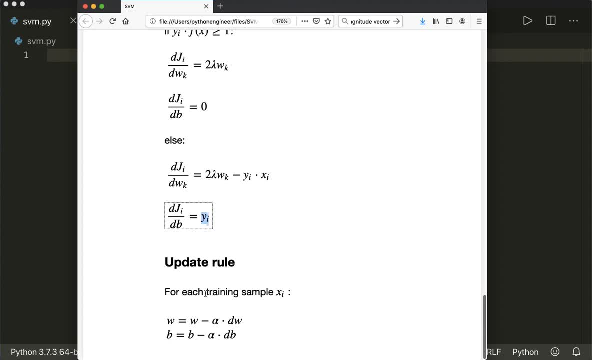 then, when we have our gradients, we can use the update rule. So the new weight is the old weight, minus because we use gradient descent, so we go into negative direction, minus the learning rate or the step size times the derivative. So these are our gradients And 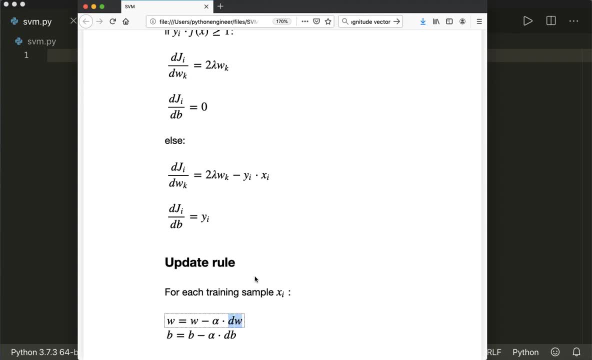 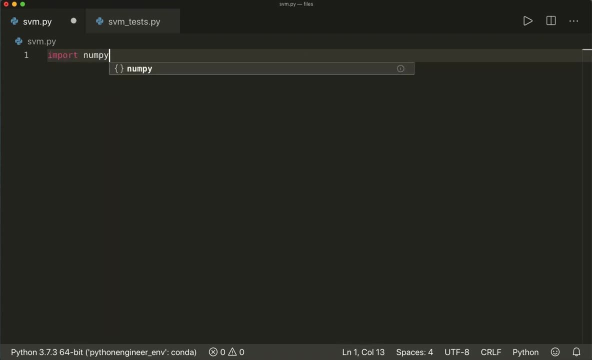 then the derivative. So these are our update rules, And now I hope you've understood the concept and the math behind this, And now we can start implementing it. So this is now straightforward. So first of all, we import numpy s and P, of course, And then we create our class SVM, which will 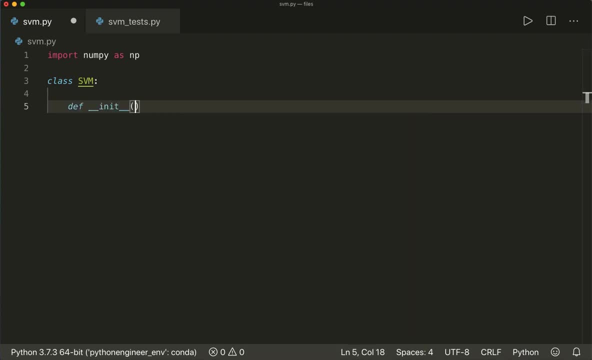 get an init method, And here I will put in a learning rate which will get a default value of point zero, zero one, And it will get a lambda parameter which will also get a default, and I will say: this is point zero one. So 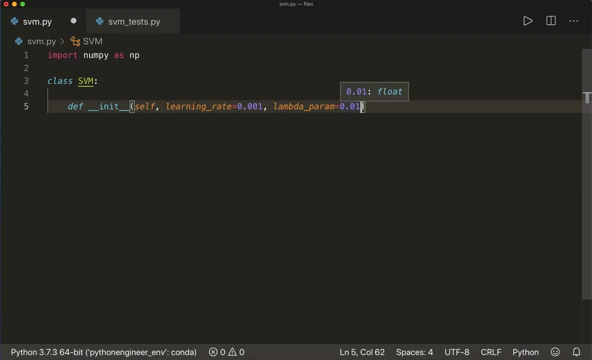 this is usually also a small value, And then it will get the number of iterations for our optimization, which will get the default of 1000. So then I will simply store them. So I will say: self dot l r equals learning rate. self dot lambda param equals lambda param. So note that I cannot use lambda here, because 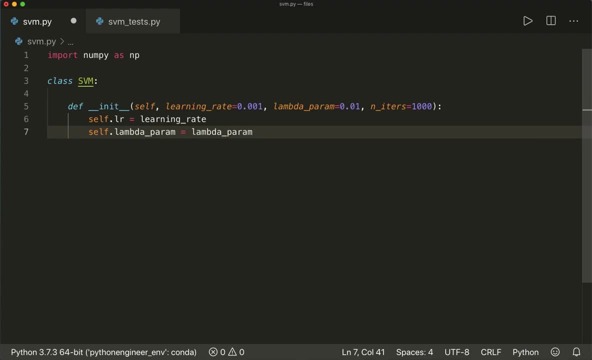 lambda is a keyword in Python for the lambda function. So yeah, then self dot n- Ethers equals and editors. then I will say self dot w equals none and self dot b equals none. So I have to come up with them later, And then we define our two functions. So, as always, 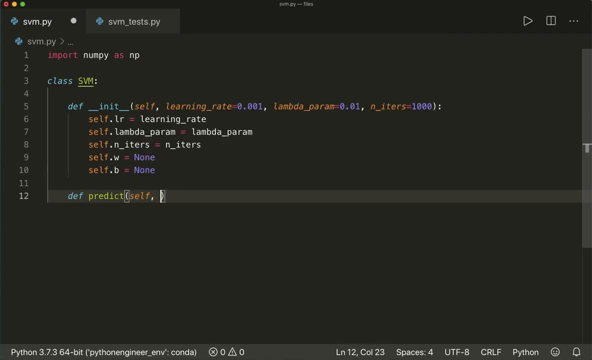 one is the function, where we fit the training samples and the training labels And the Sorry. this is the fit method, And the other one is the predict method, where we predict the labels of the test samples. And now let's start with the predict method, because this is very short. 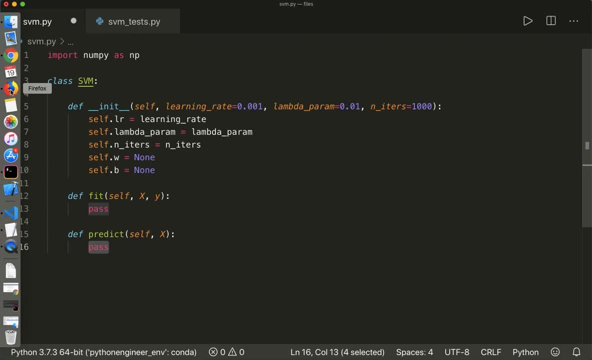 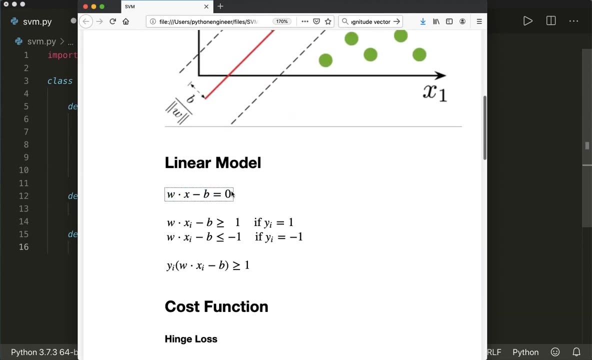 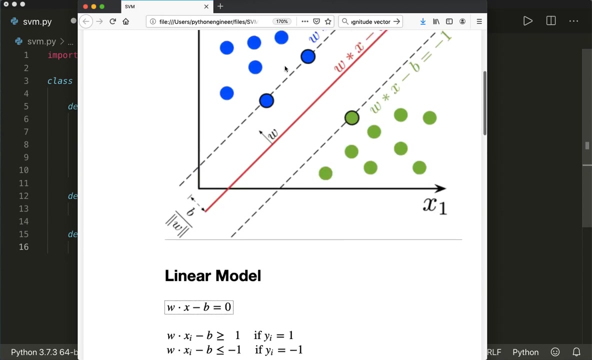 So we want to, as I said, if we look at the math, we apply this linear model and then we look at the sign of this. So if it's positive, then we say it's class one, And if it's negative, 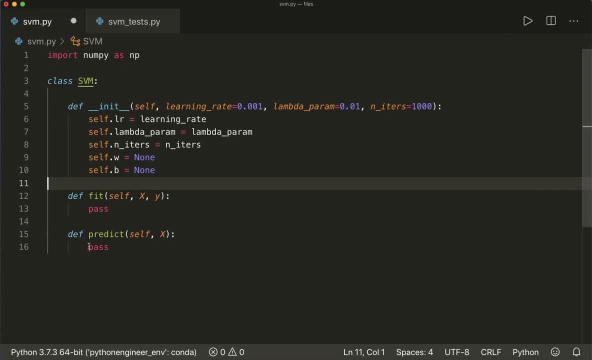 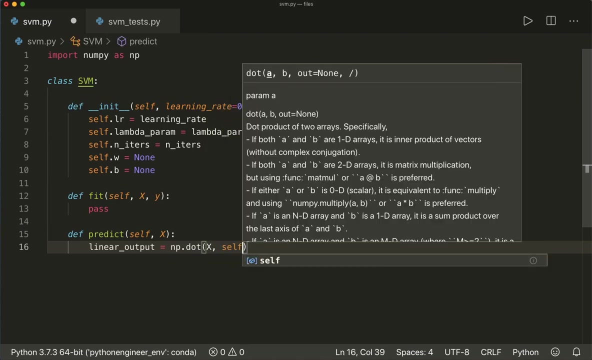 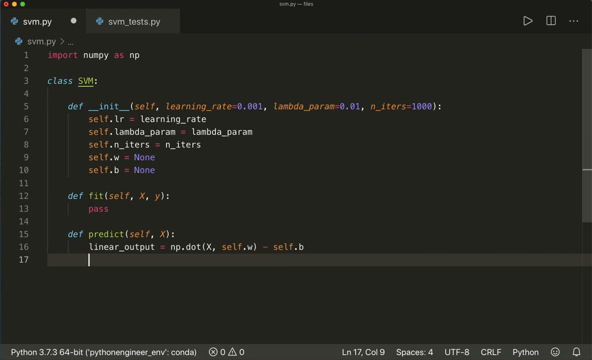 then we say it's class minus one. So we say linear output equals number: pi, dot dot. so the dot product of x and self dot w minus self dot b, And then we choose the sign, so we can simply say: return numpy dot sign of this linear output. So this is: 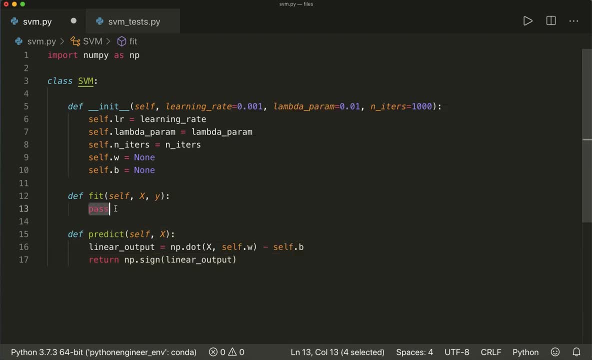 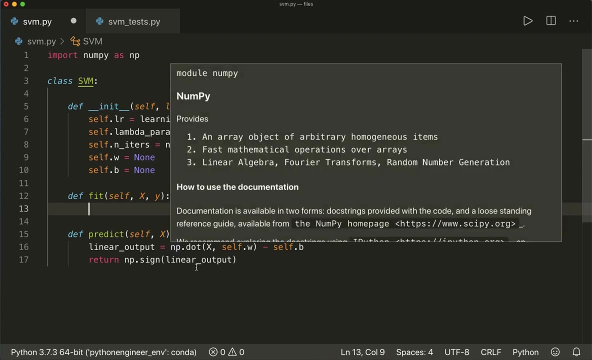 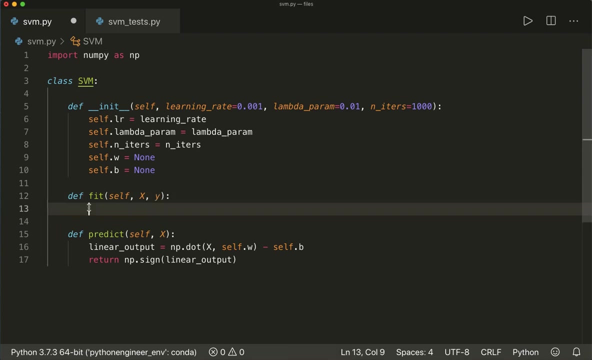 the whole predict implementation. And now let's continue with the fit method. So first of all, as I said, we use the classes plus one and minus one here, So we want to make sure that our y has only minus one and plus one, So oftentimes it has zero and one. So 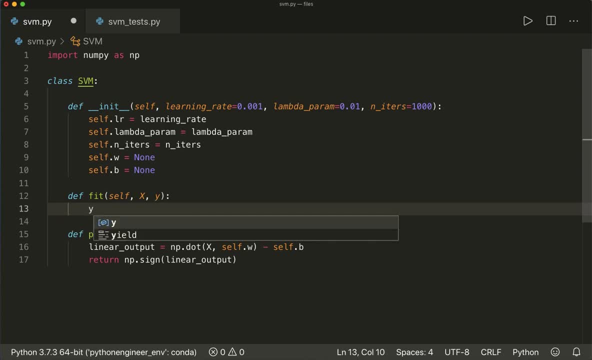 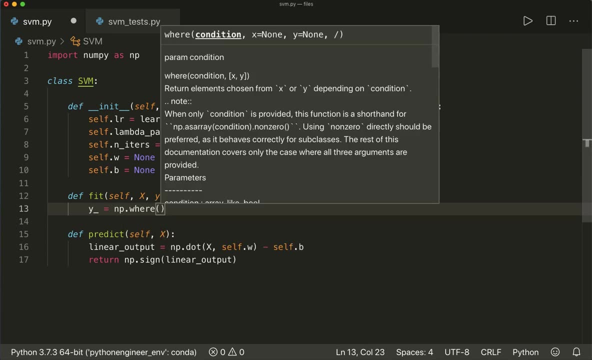 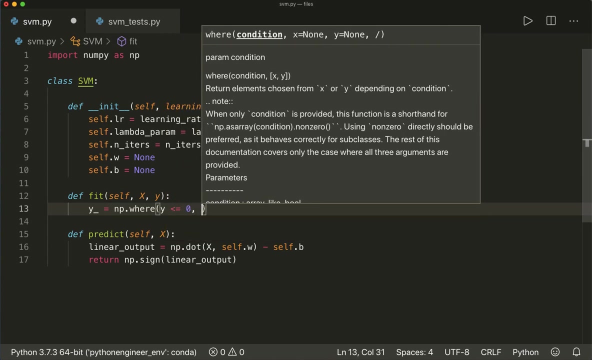 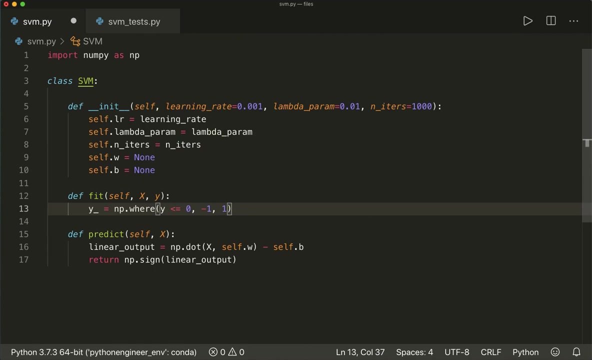 let's convert this. So let's say y underscore equals, And here we can use numpy dot, where this will get a condition. So we say why if this is less or equal than zero, then we put in minus one, and otherwise we put in plus one. 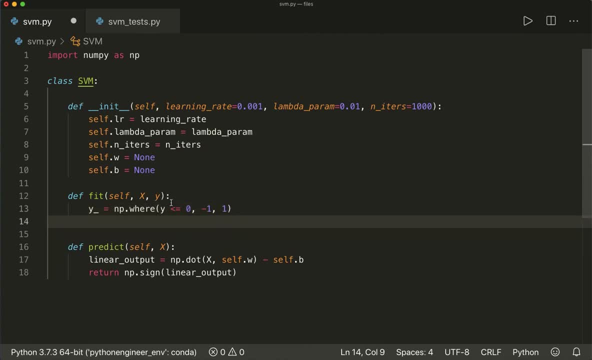 So this will convert all the zeros or smaller numbers to minus one and the other numbers to plus one. And now let's get the number of samples and the number of features. And this is simply x dot shape, because our input vector x is an numpy nd array where the number of rows 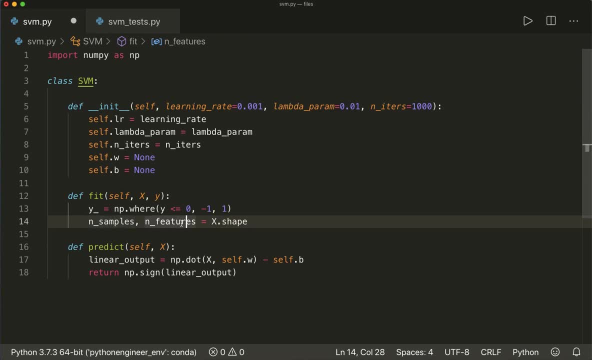 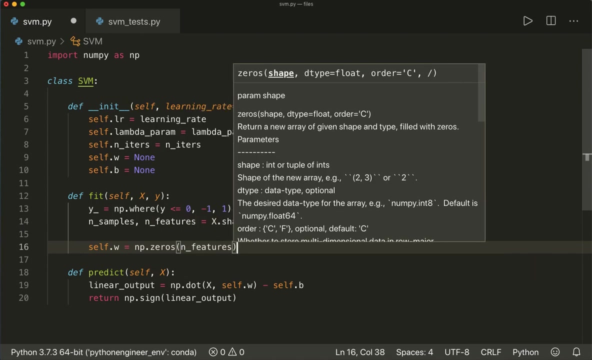 is the number of samples and the number of columns is the number of features. then we want to initialize our w and our b And we simply put in zeros in the beginning. So we say self taught w equals non pi, zeros of size and features. So for each feature component we 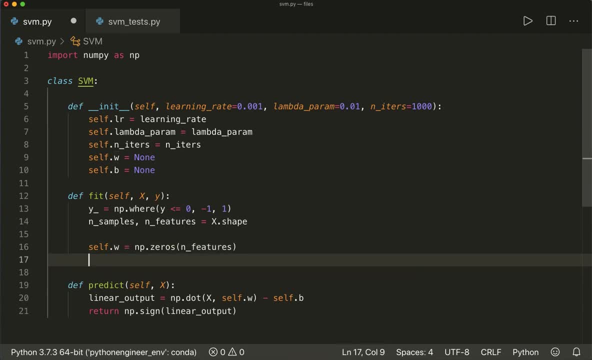 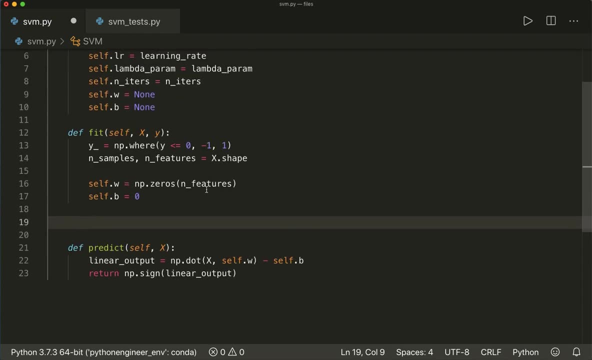 put in a zero for our weight component And then we say self dot B equals zero And now we can start with our gradient descent. So we say for underscore, because we don't need this in range self dot and it iterates. So the number of iterations we want to do this. 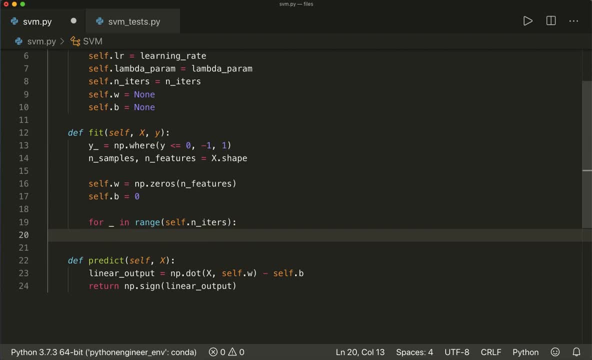 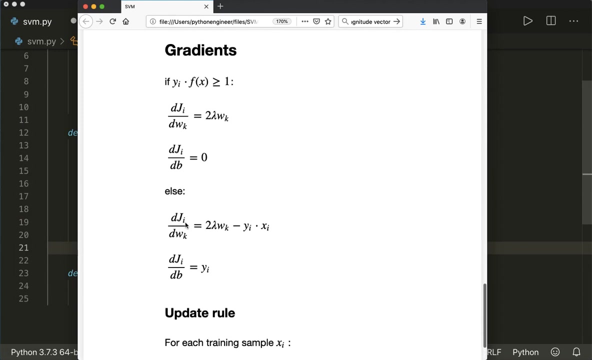 And then we iterate over our training samples. So I say, for index and x, i in enumerate x. So this will give me the current index and also the current sample. And now, what I want to do now is let's have a look at the math again. So I want to come, I want to calculate the weights. 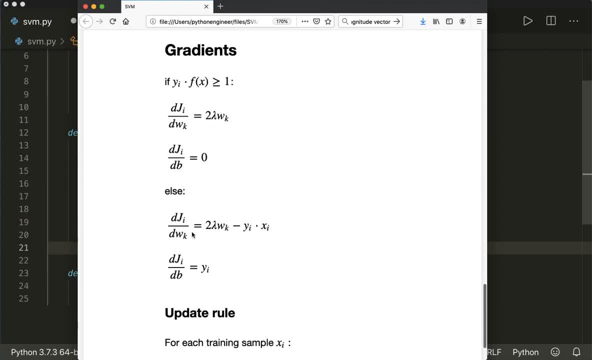 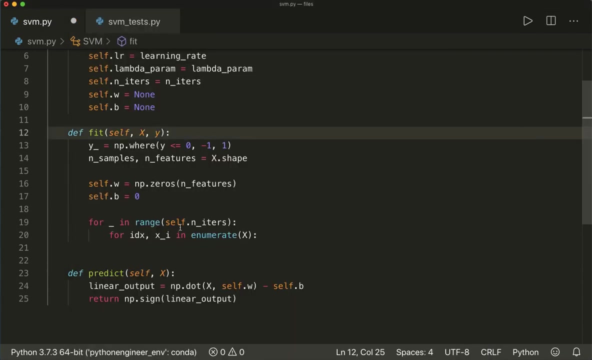 at the derivative of our cost function with respect to the W and with respect to the bias. And here I first, but first I look if this condition is satisfied. So I will say: and the condition is y i times our linear function. So I say condition equals y underscore of the current index times. 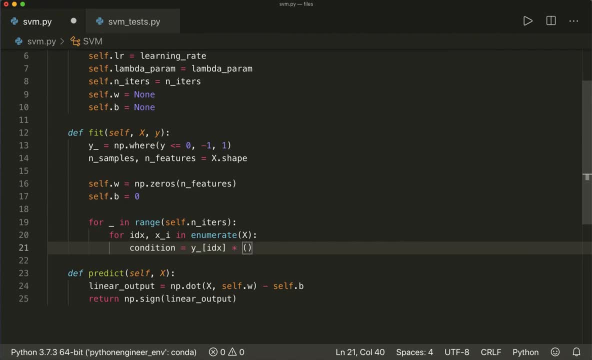 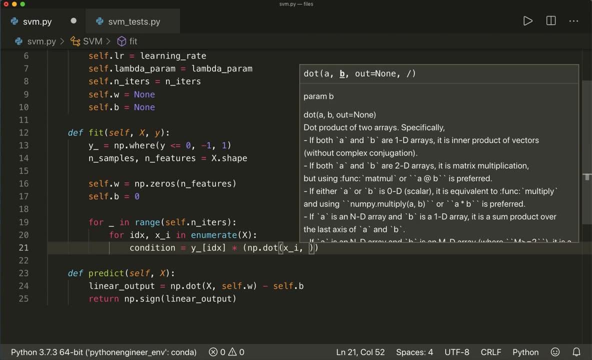 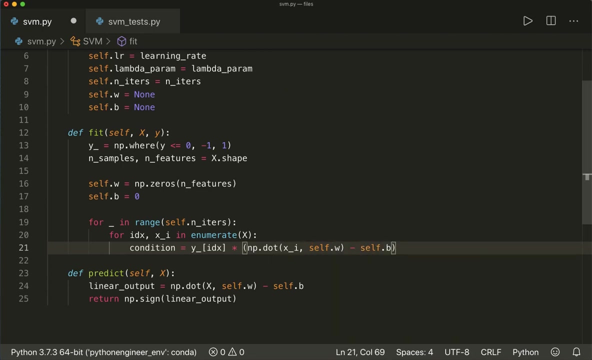 and then the linear function, So numpy dot of the current sample and our self dot w minus self dot b. This should be greater or equal than one. So if this is satisfied and the condition is true, and otherwise it's false. So now I say if condition. so if this is true, 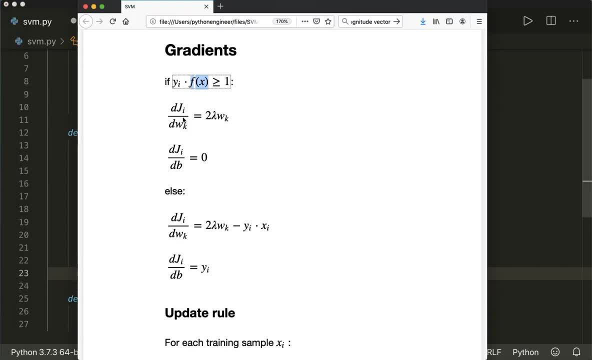 then our derivatives look like this: So the derivative with respect to the B is just zero, And so we only need this. So I say so it's two times lambda times w. And then in our update we go in so we say: 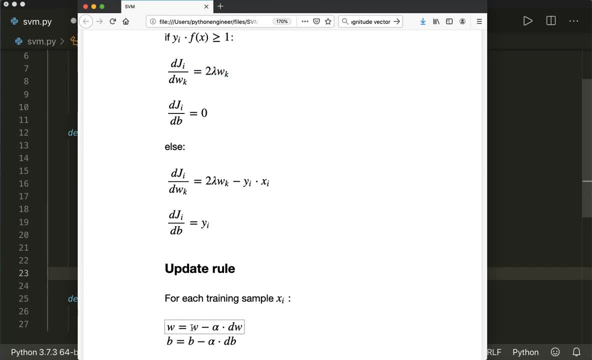 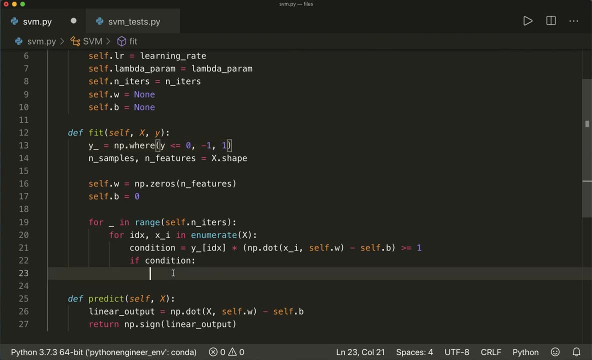 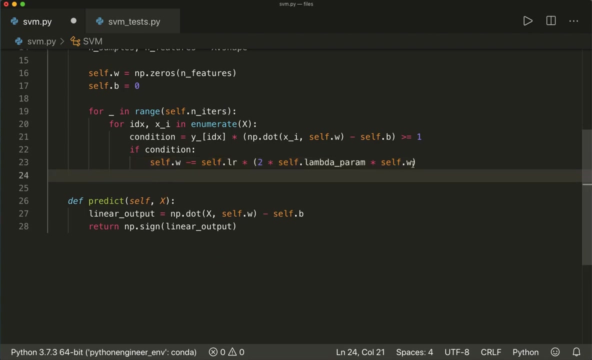 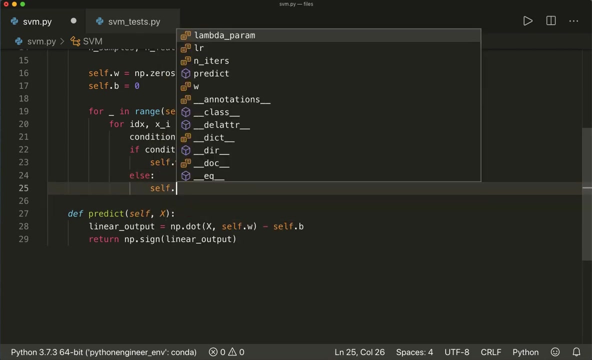 q dot lambda, subref. P R Sonic times y i DC payment. And then we write: Benjamin times, self dot w. So this is the first update, or if our condition is satisfied and we only need this update And otherwise we say: self dot w minus equals self times. l? r the learning rate. 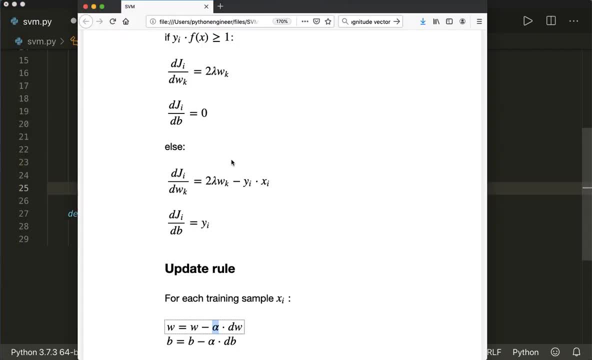 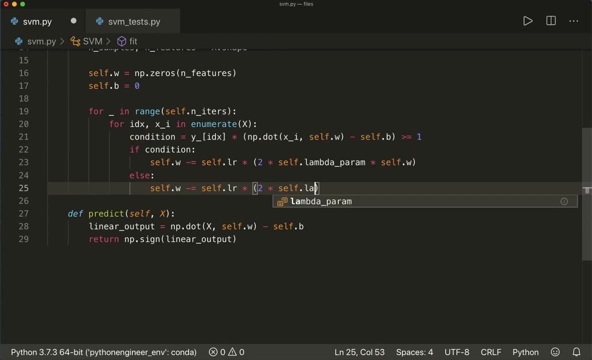 times. And let's again have a look at the equation. So it's two times lambda times w minus y i times x- i. So two times our lambda times the w minus numpy dot. so I want to multiply our vectors x, i and. 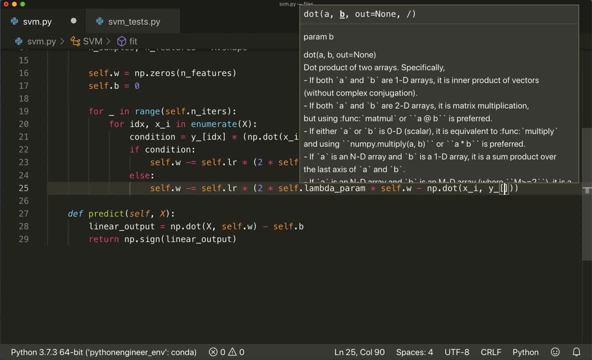 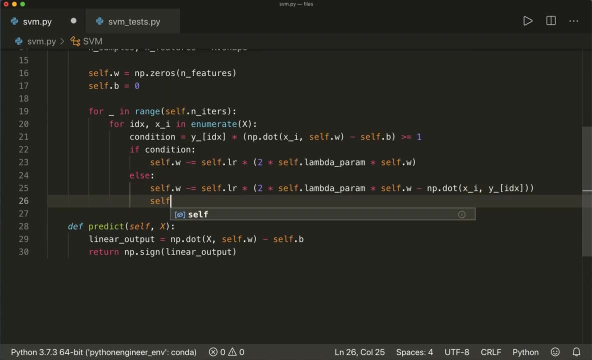 y, i, so the y underscore of the current index. So this is our update for the w and our self. dot b is minus, equals self times, learning rate times. the derivative and the derivative is only or just y, i, so only y underscore of the index. 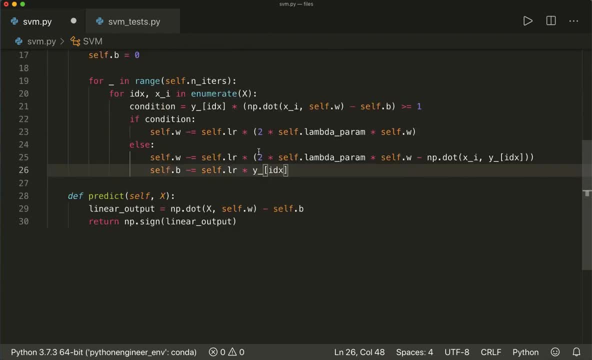 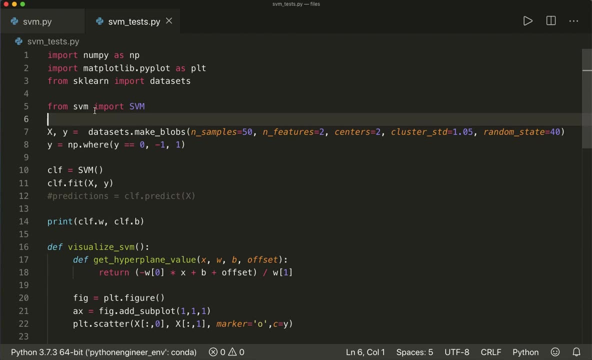 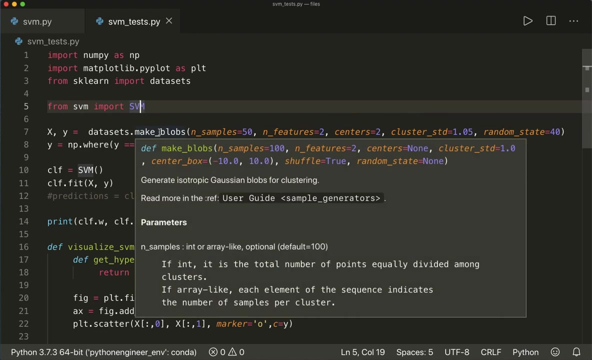 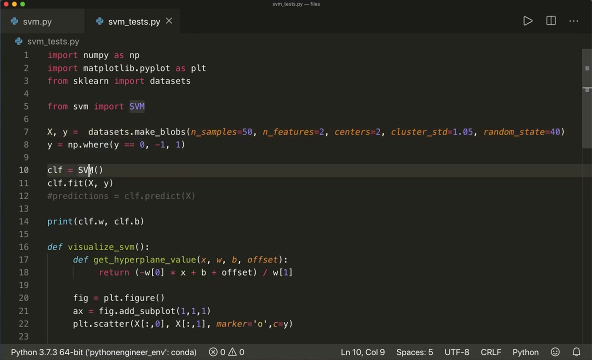 And now we're done. So this is the whole implementation, And now let's test this. So I've written a little test script that will import this SVM class And then it will generate a some test samples. So it will generate two classes And then I will create my SVM classifier and fit the data. 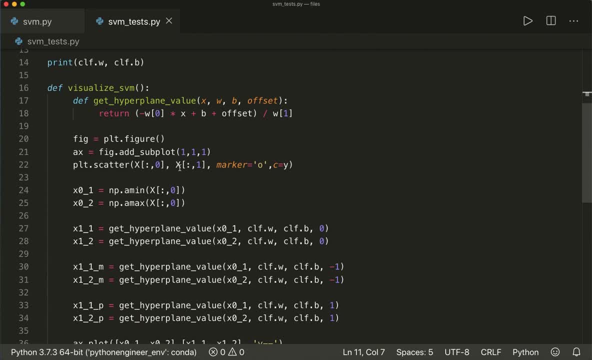 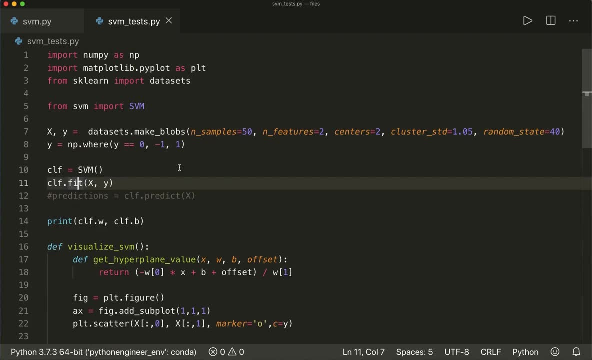 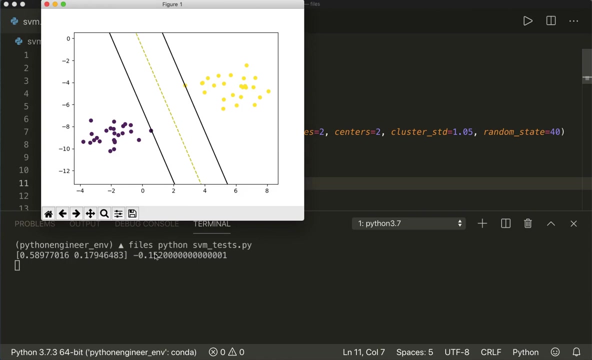 And then I wrote a little function to visualize this, So you can find the code on GitHub, by the way. So please check that out for yourself. And now, if we run this, so let's say Python, SVM, underscore, test, dot, pi, And now this should calculate the weights and the bias, and it should also.